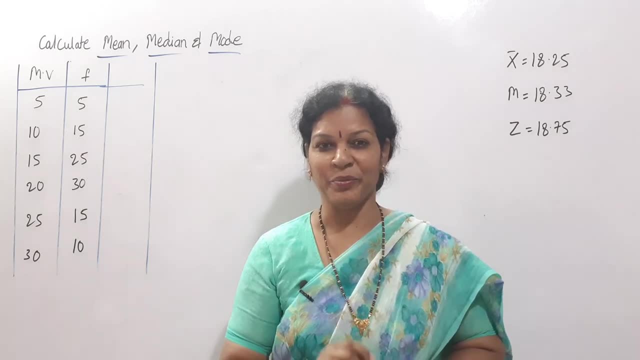 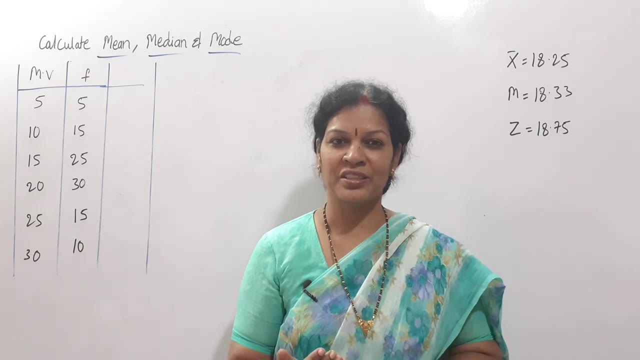 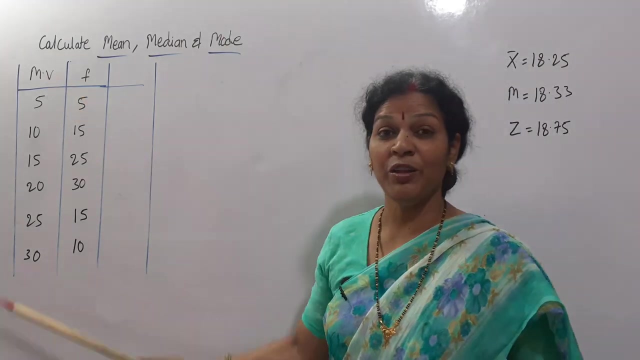 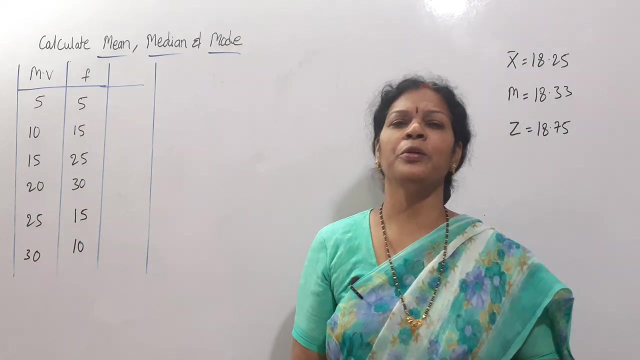 In exams nobody will ask you to calculate median, calculate mean. They will ask you to calculate three together. So that is why I will make your practice of working out this in one problem. Now see the problem: Calculate mean, median mode. What is the data given to us? Mid value is given, not x. Mid value is given frequency. First of all, mid value, we have to turn it into x. That we will do first. 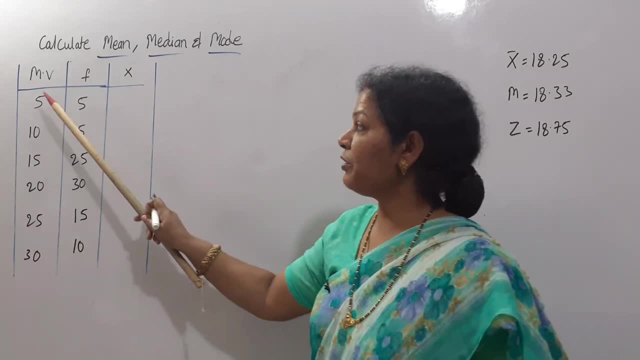 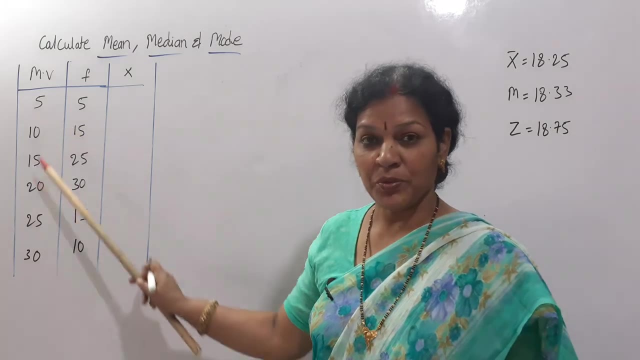 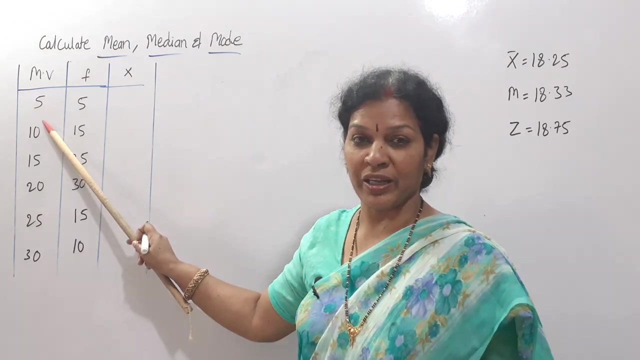 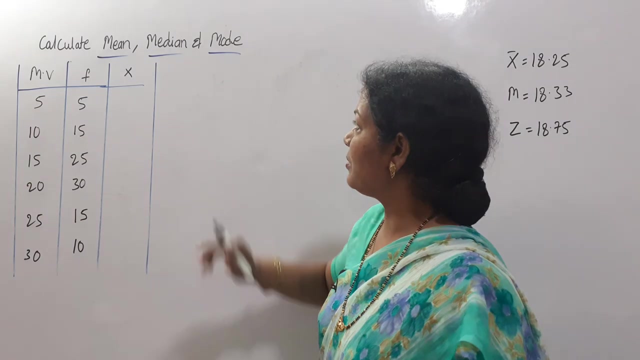 X How to take Mid value difference, any difference if you take phi Phi divided. already I taught you this one Difference is phi Phi make it half means 2.5.. 2.5 if you deduct from phi, you will get lower class interval. If you add to this phi, you will get upper class interval. So the difference is here. phi Phi, make it half divided by 2 means 2.5. 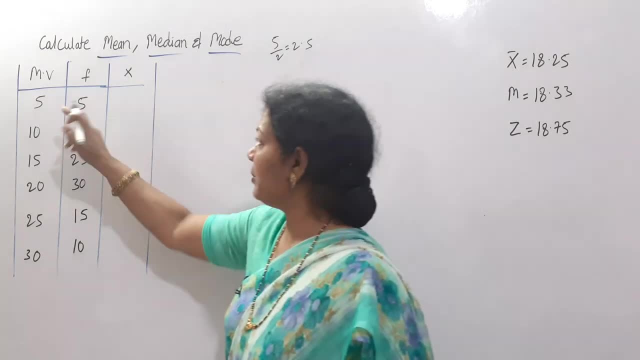 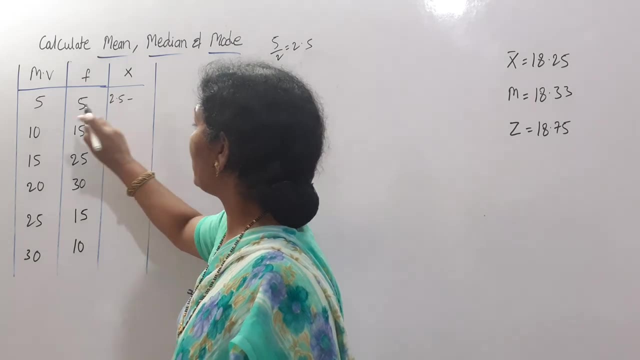 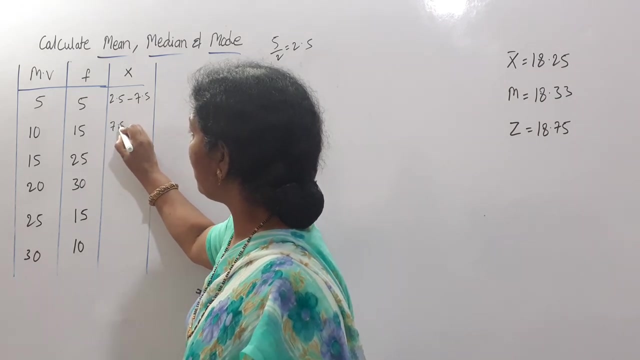 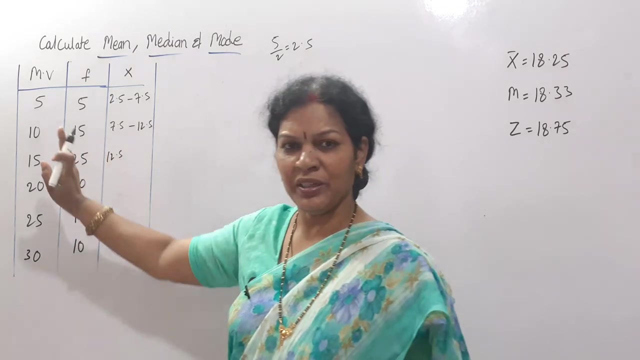 2.5. if I deduct From this, I will get lower class interval. Means, if I deduct from this, phi minus 2.5, 2.5.. 2.5. If I add 2.5, upper class interval, that is 7.5.. In the same way, here also 7.5 and 12.5.. Here, 12.5.. What we are doing, Deducting 2.5, we are getting lower class interval, Adding we are getting upper class interval. 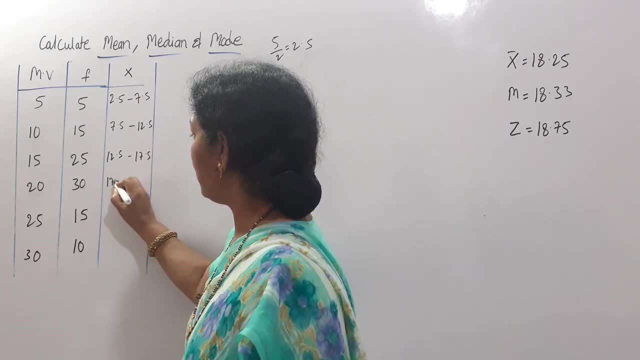 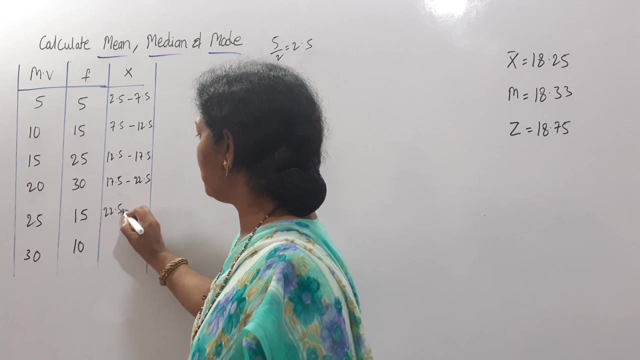 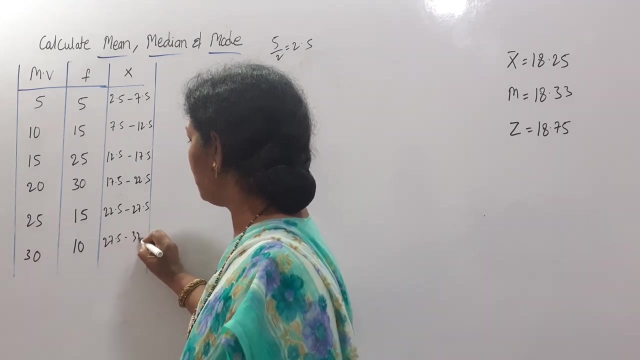 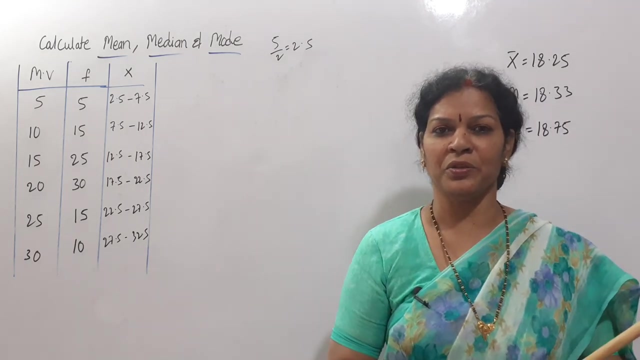 2.5 to 17.5.. 17.5 to 22.5.. 22.5 to 27.5.. 27.5 to 32.5.. Like this you got the class interval X Problem. I am not going to work out, You have to work out. I will explain you. That is it. 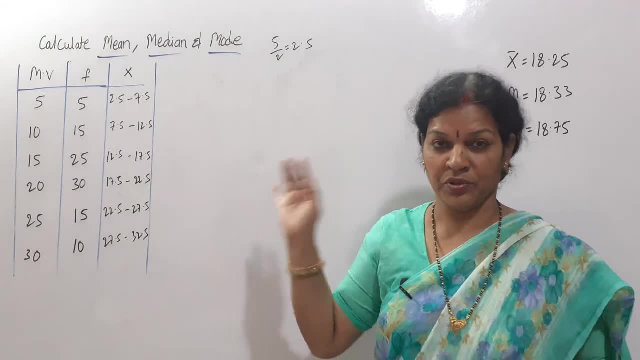 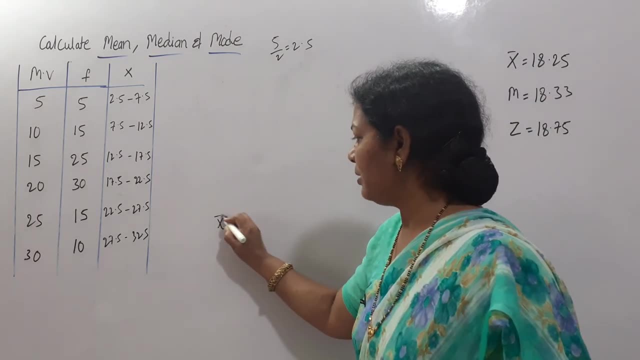 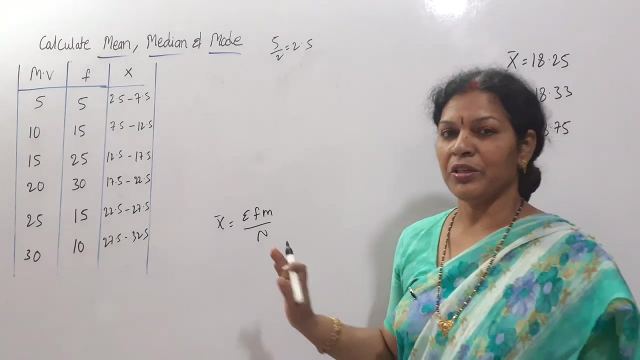 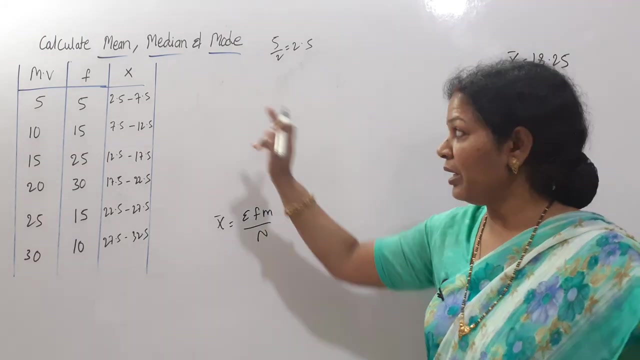 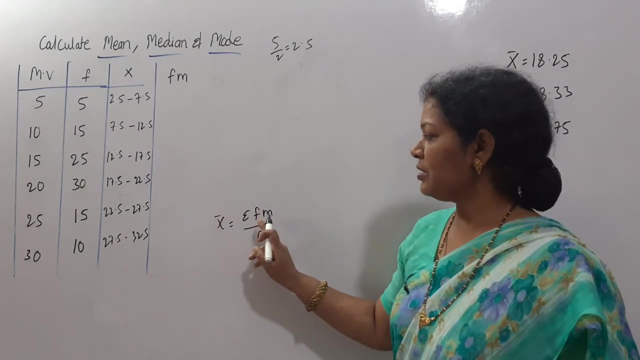 First of all, whenever you find this mean median mode, Find what are the formulas. X mean formula. What is the formula? mean X bar is equal to sigma fm by n Formula. you got it According to that. what do we need? First of all, mid value, Mid value already, given. What else is needed? Frequency into mid value. So I will provide one column: frequency into mid value. This I will get. Total of this is sigma fm. 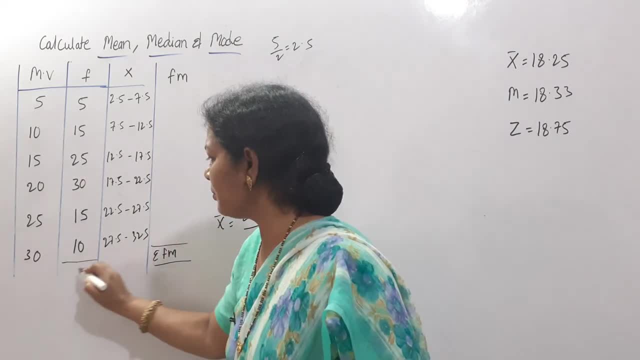 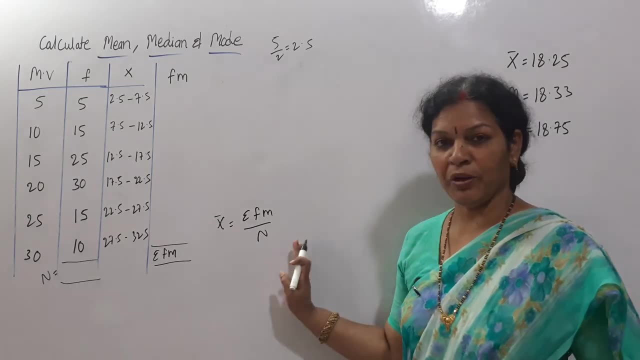 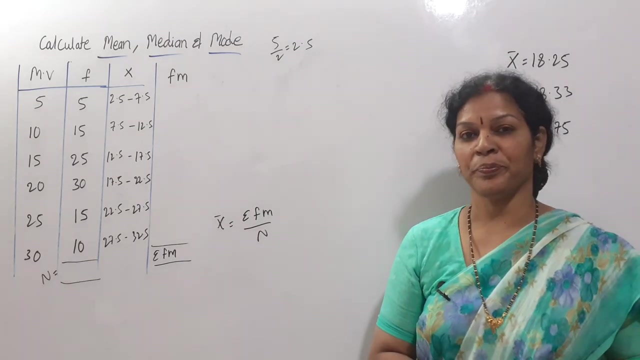 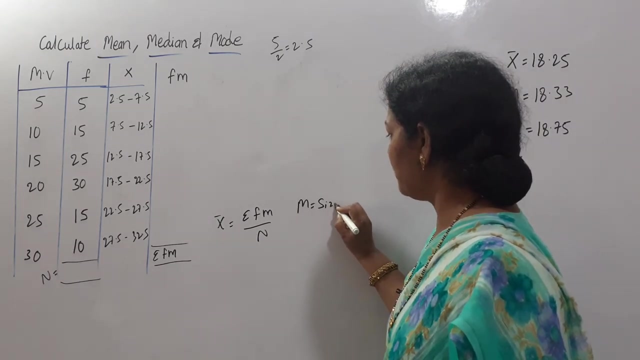 N is total of this frequency Columns. I have Fm. I will calculate, Put it in the formula So that I will be getting the X bar. That is arithmetic mean value. Mean is over Next median Median. What are the two formulas? are there? First formula is: median is equal to size of n by 2. th item: 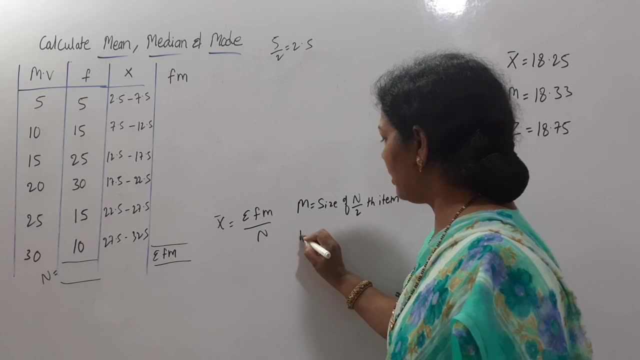 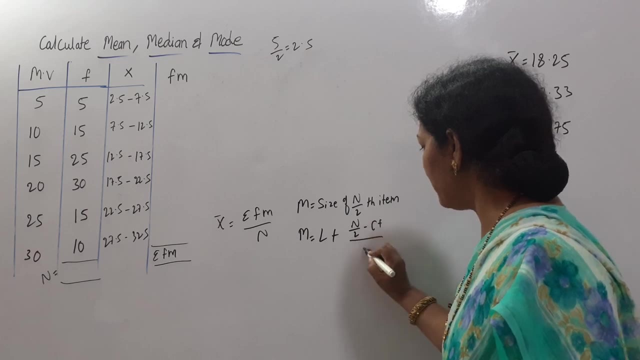 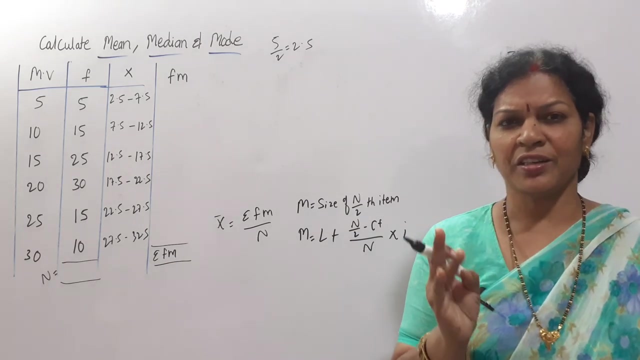 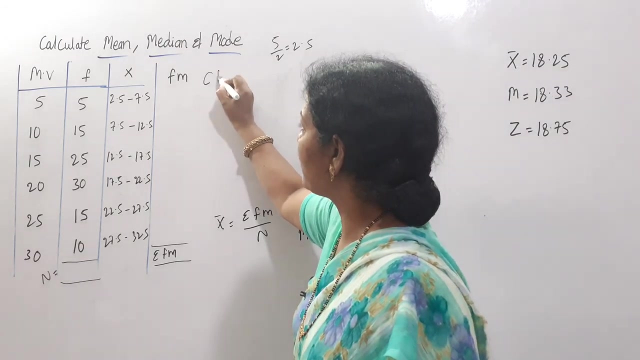 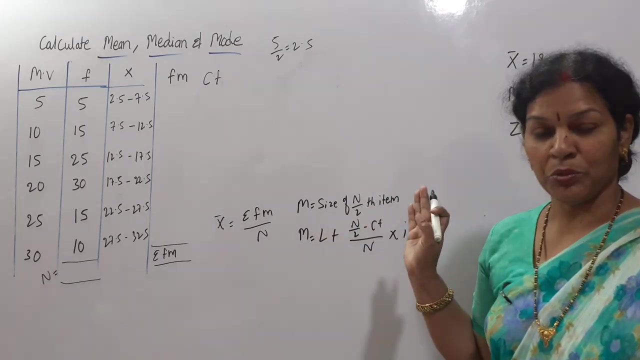 And what is the second formula? Second formula: m is equal to l plus n by 2, minus cf by n into i. This is the formula Right. Whenever you want to calculate median, Either in discrete series or continuous series, Immediately, first thing what you have to do is cf, Cumulative frequency. you have to calculate. So I will provide a column for cf. Only this column is enough Cf you will get. Then you will apply the n by 2. th item: 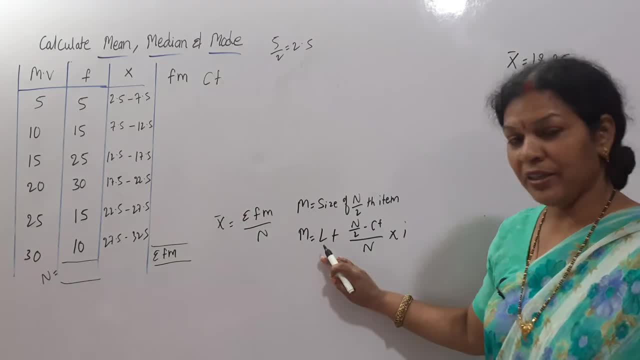 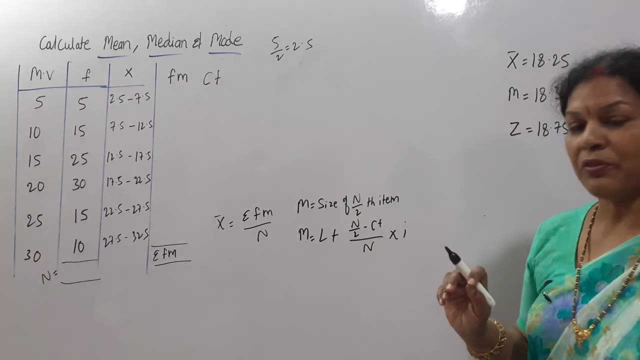 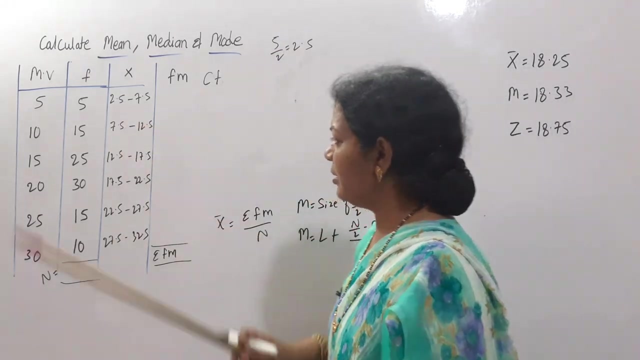 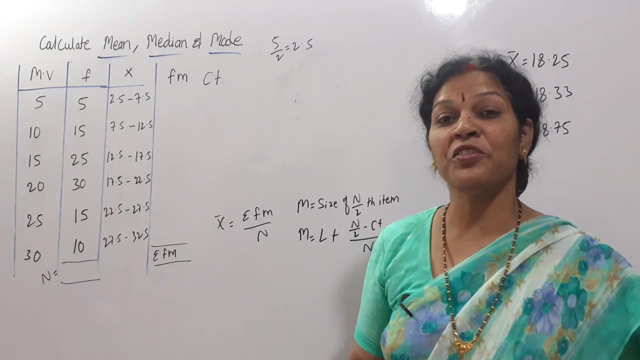 Then you will get license cf, You will identify the class interval And you will apply this formula We have done already, Okay? So like this median, you are going to find out Next after that, mode Mode For mode, If you see the frequency, Highest frequency is 30.. Next highest is 25.. There is a difference. So that is why by inspection mode lies in so and so class interval. You can write one sentence. So this is mean. 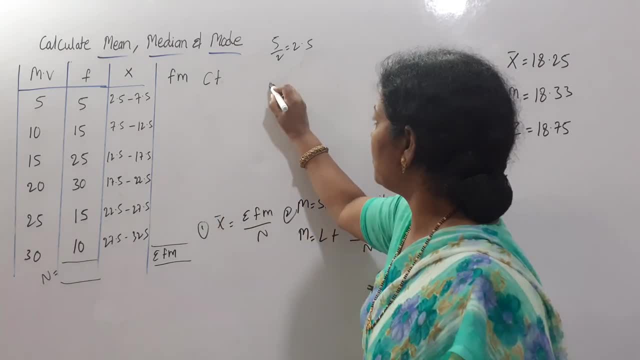 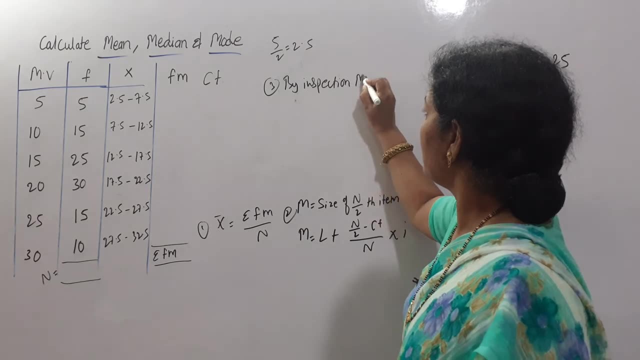 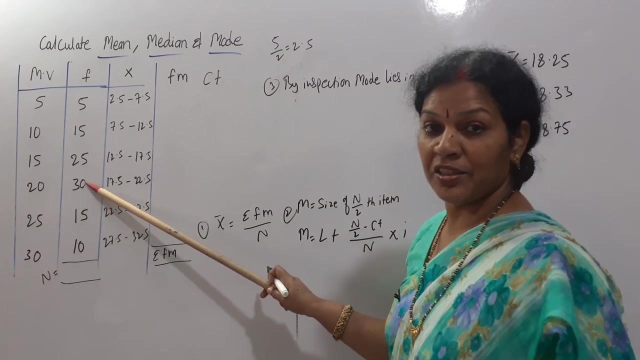 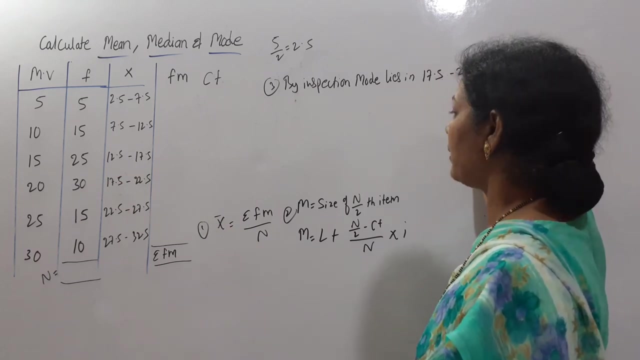 Median. And coming to mode, You can write by inspection. Mode lies in Which class interval? here 30 is the highest frequency, So mode lies in 17.5 to 22.5.. Yeah, 22.5. Okay. 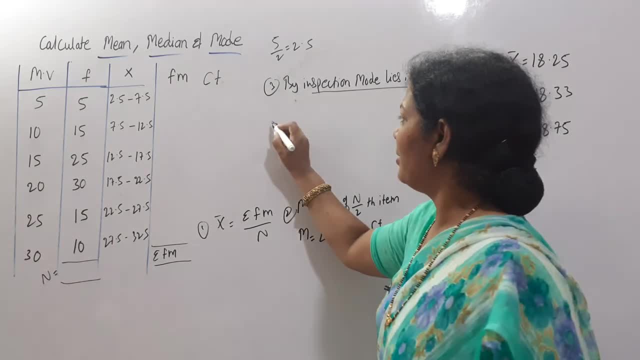 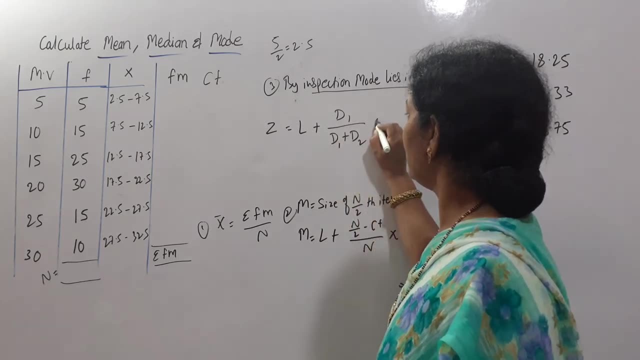 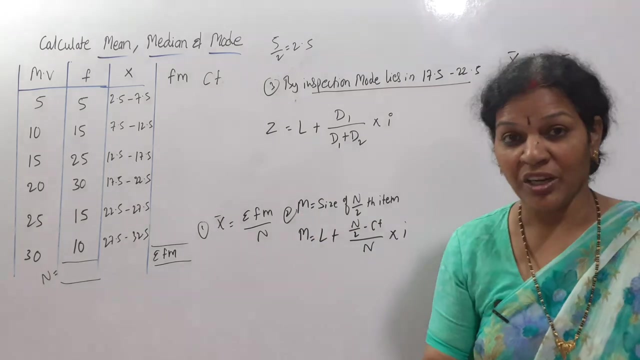 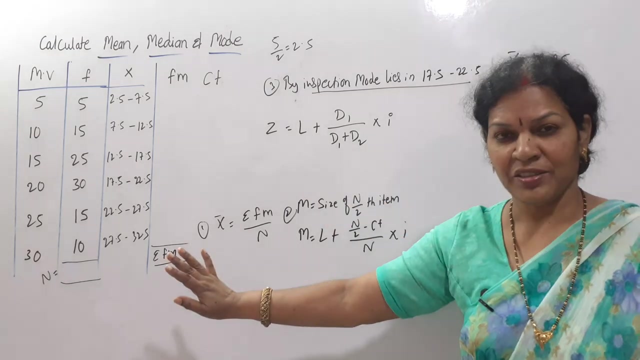 Then after that write the formula. What is the formula? Did you remember? Mode formula is l plus d1 by d1 plus d2. into i Apply this And you will get mode also. So this is your homework problem. I am not going to work out because we have done enough problems. Just in one glance. I explained you how to prepare mean median mode. Do not get confused.